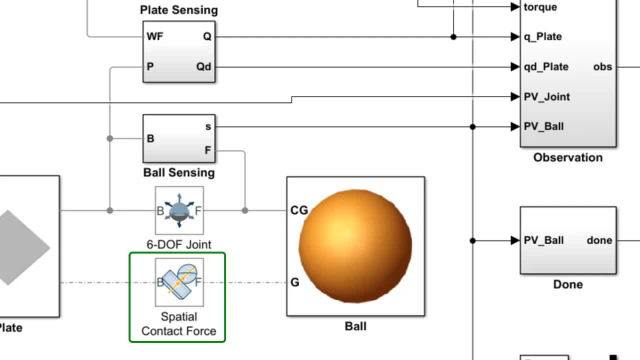 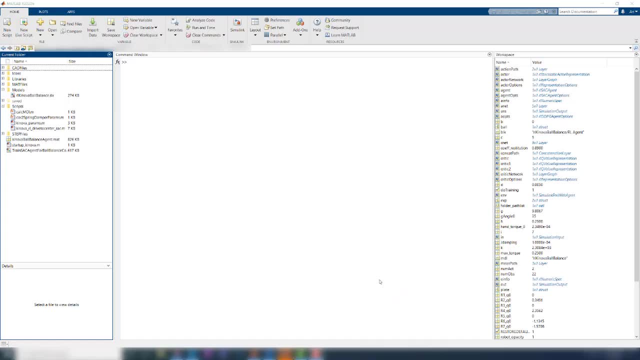 The contact force between the ball and plate is modeled using a spatial contact force block which basically behaves like a spring and mass temper system. Now we can look into each of the subsystems to understand them better. In the project folder you can find the Simulink model under the models folder over here. You 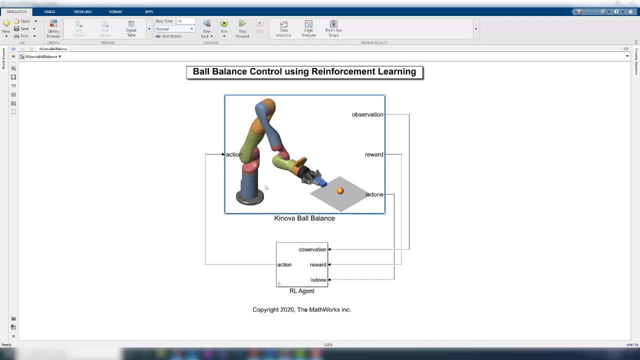 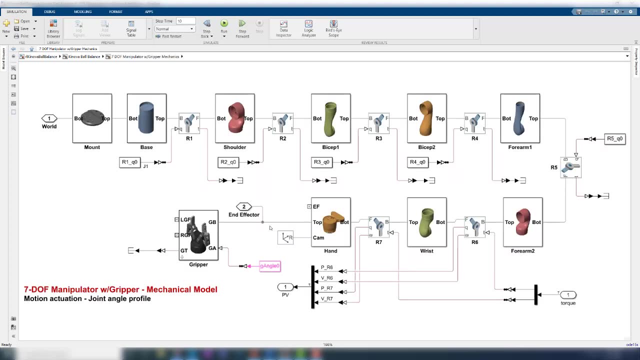 can open the model and once the model is open, you can navigate under these subsystems and look at them with more detail. In the robot subsystem we see the different parts of the robot arm, where the links and joints are represented by Simscape multi-body blocks. These components were created by importing the 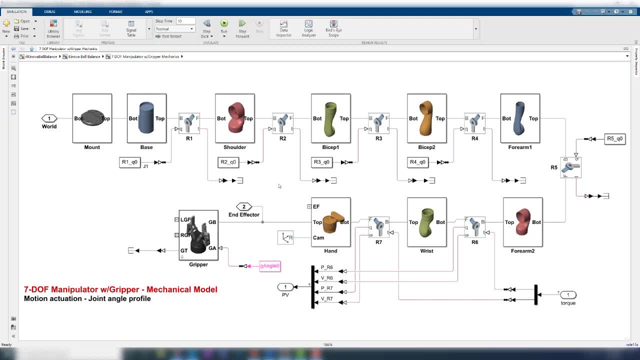 CAD geometries or step files using the SM import command. We won't go through the import workflow in detail, but you will find more information on this towards the end of this tutorial. The Revolute joints- the Revolute joint blocks- are responsible for motion between the links, and the motion is computed after. 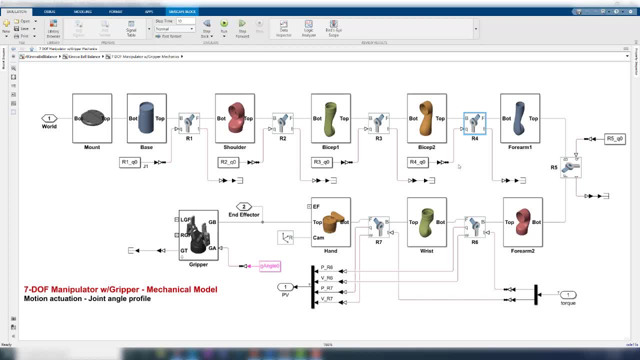 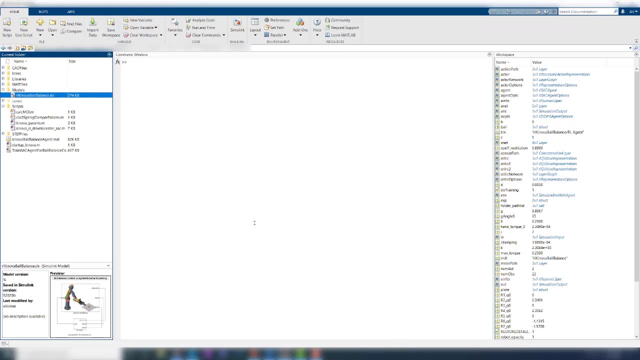 injecting torque signals into the revolute joints. For this example, we make it simple by only actuating the last two joints, which is the R6 and R7 joints, over here. The other joints remain static at some predefined joint angles. These angles are specified in an initialization script that you can find over here. You can open. 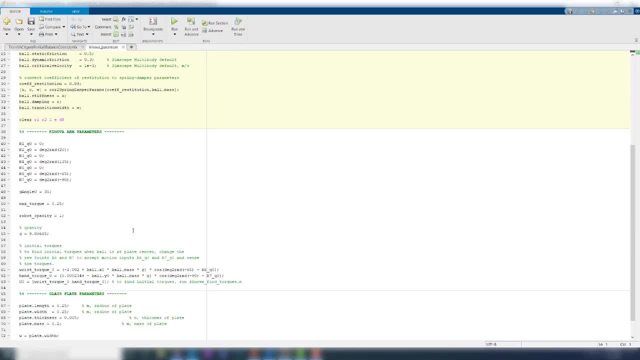 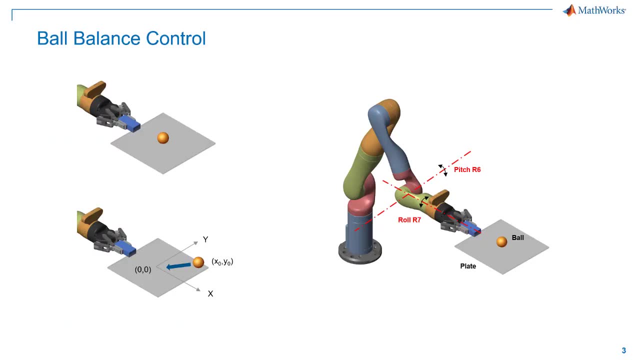 this script to view the different parameters of the system, and feel free to change anything you like over here. After getting familiarized with the model, let's take a look into the control problem. In this example, the task is to balance a ping-pong ball on the plate At. 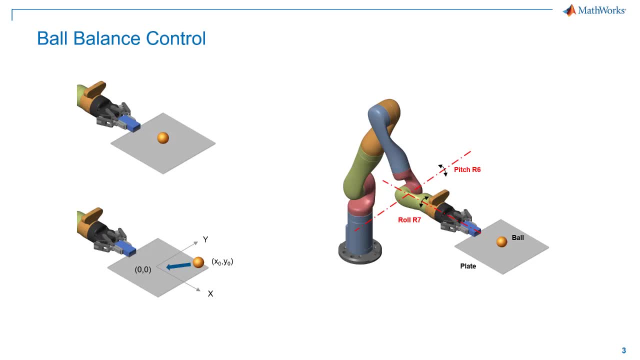 the beginning of our simulation. the ball can start from any location within the plate and the control algorithm should calculate the necessary torque signals to drive the ball to the center and balance it over there. This task can be solved using popular control algorithms like MPC or other optimal control. 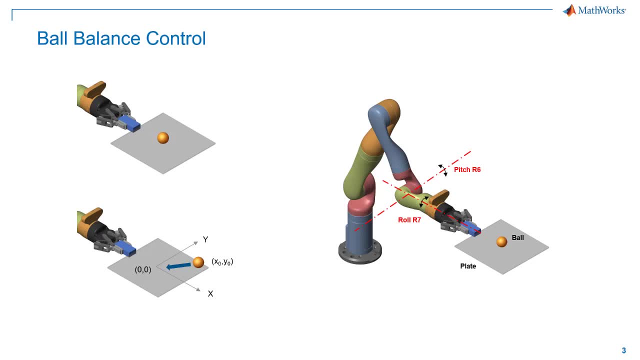 methods. However, because we need a mathematical model of the plant for such algorithms, designing controllers may become difficult when the system is complex. For example, if you were to design an MPC controller for the entire system by actuating all joints, you would 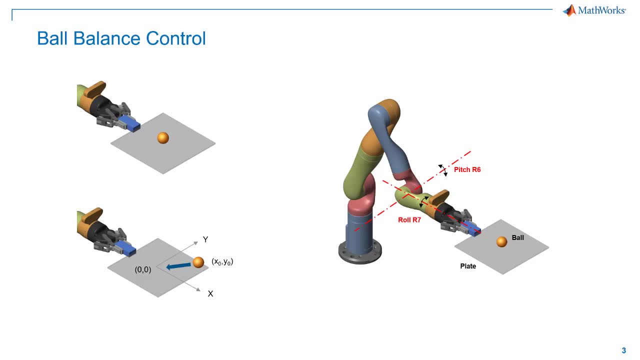 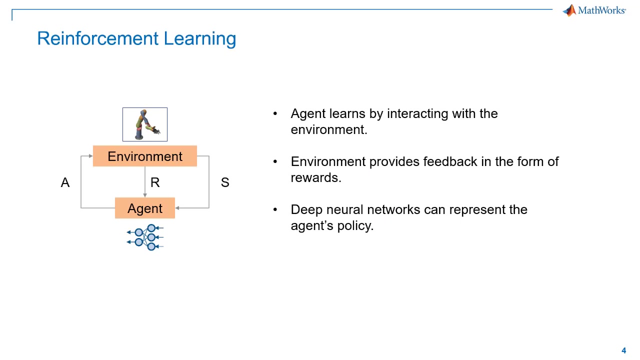 need to compute Jacobians or write a transition function for the dynamics, which could be a tedious process. This is where reinforcement learning can provide an alternate method for designing controllers. Here is a quick overview on some key concepts in reinforcement learning. We will focus on the section of 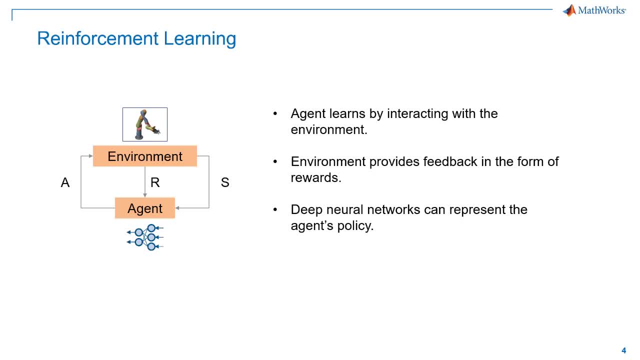 reinforcement learning that is known as model-free reinforcement learning. as the name suggests, The algorithm does not need a model of the plant. Instead, the desired behavior is learned by the system itself. The model results can be used to by repeated interaction with the plant. this diagram shows the standard data flow in a. 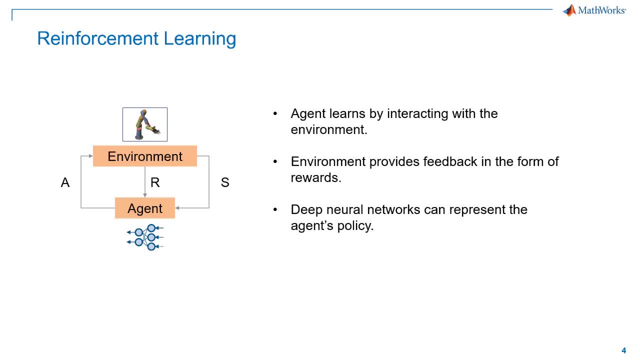 reinforcement learning setup. the controller in the setup is the RL agent, and the remainder of the system, including the, including the robot plate, the ball and their actuation and sensing components, is known as the environment. the agent interacts with the environment by providing a set of action signals, which is represented by a, and the environment uses these signals to step into. 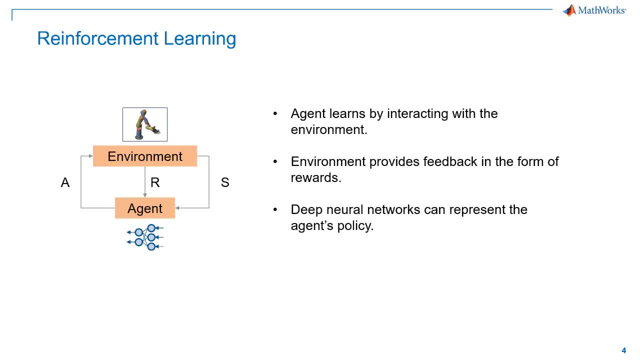 the next state s which is rendered done to the agent. the agent also receives another signal R from the environment, called the reward, which is a feedback on how well the choice of action was suited for the control task. the goal of the learning algorithm is to maximize this reward. 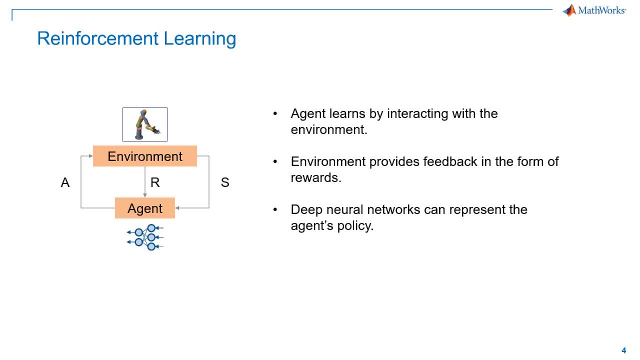 over time to repeated interaction of the agent and environment. in this tutorial we will represent the agent using deep neural networks. you can find more information on designing neural networks in the MATLAB documentation or on our website at matlabcom. but for now, let us see how we can use the reinforcement learning toolbox to solve the problem. 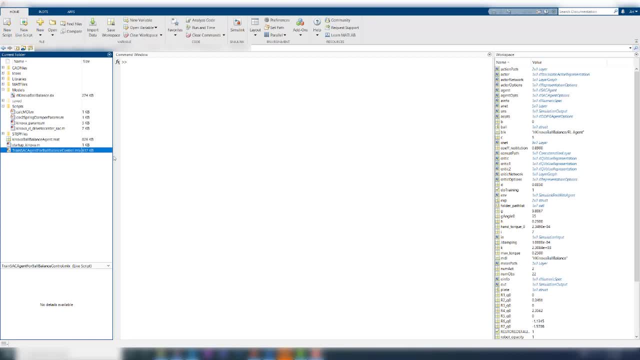 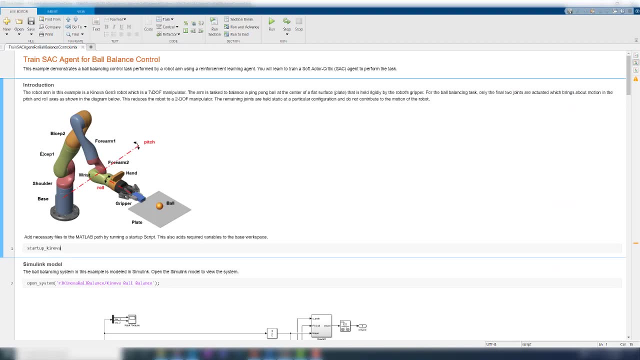 when you are back in the MATLAB window, open the live script from the project folder here. this script contains a standard command line workflow for reinforcement learning. we begin by running a startup script which adds the necessary files to the MATLAB path and creates the required variables in the base workspace. to run the script, you can click on the 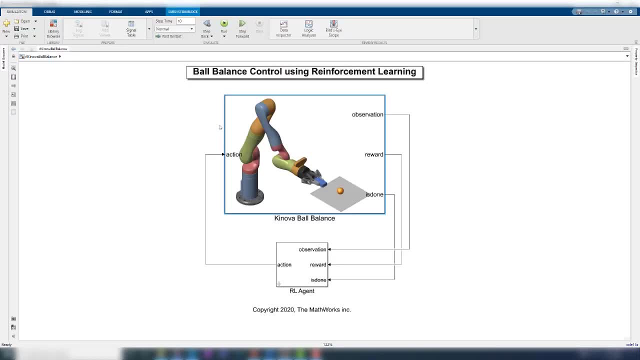 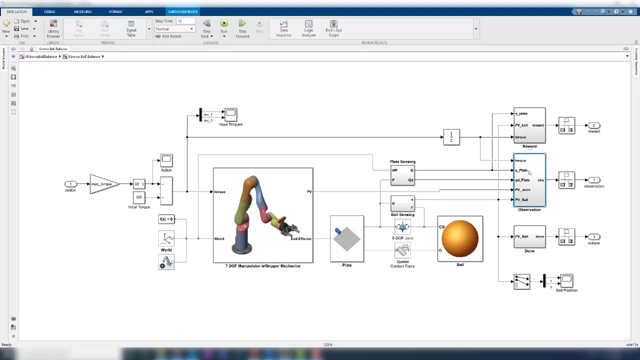 script to run the script and this also opens the simulink model. at the top level of this model, you will see the reinforcement learning setup that we discussed earlier with the agent exchanging data with the environment. let's navigate into the environment and open the observation subsystem to. 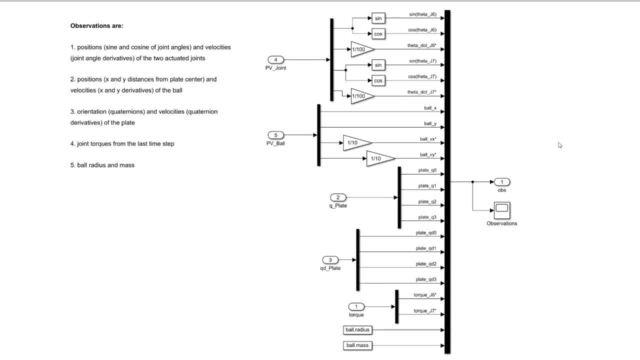 view the signals. the observation is a set of 22 signals that represents the state of the system at. It includes information on the position and velocities of the actuated joints, position and velocity of the ball, the plate, quaternions and the derivatives and the top inputs from. 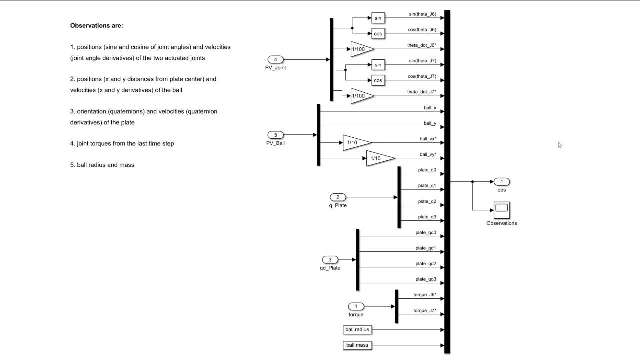 the previous time steps and then some physical parameters of the ball, like mass and radius. The agent will use these observations to compute the actions at every time step. Because these signals have different units, some of them are multiplied with these scale factors so that they remain in more or less the same range as others. 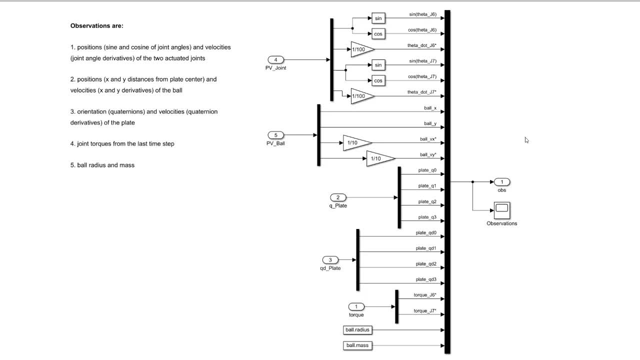 This is important because these signals will be fed into a neural network and high magnitude signals may cause one section of the network to dominate and undermine the effect of other signals. Your network will train better if you normalize or scale the observations in some manner. 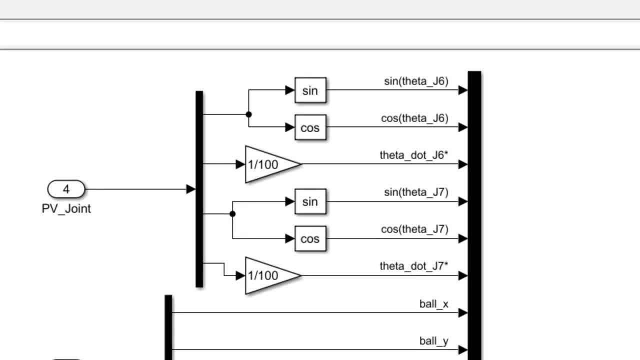 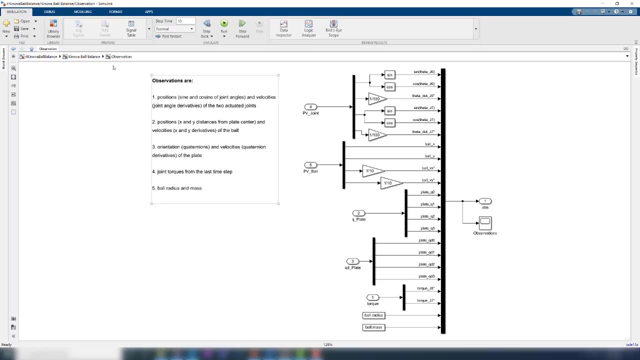 We also take the sine and cosine of the orientations instead of using them directly, in order to avoid discontinuities at the angles of plus minus pi. This is because discontinuities in the observation space may cause the learning algorithm to converge poorly. The other signal from the environment is the reward signal. 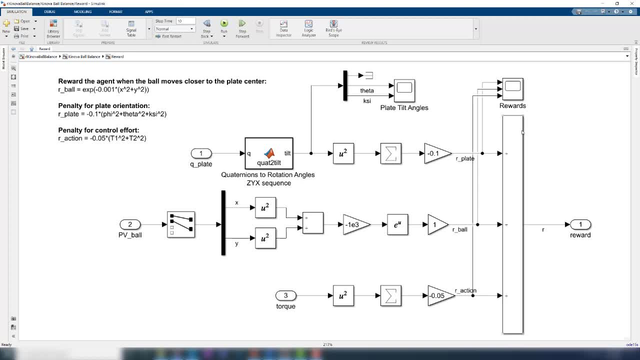 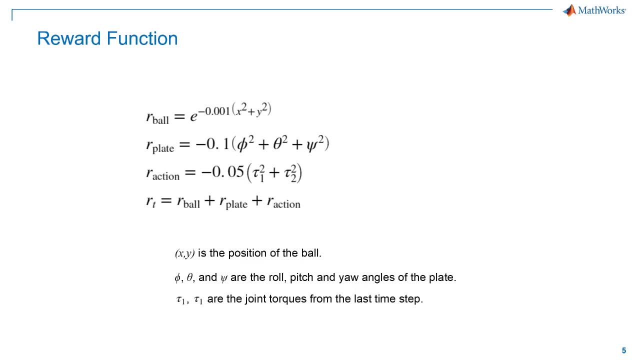 Let us take a few moments to understand the reward signal better. The reward at any time, step T- is given by the relationship shown here. Since we want the agent to move the ball to the center of the plate, we should provide a positive reward when the ball moves to the center. 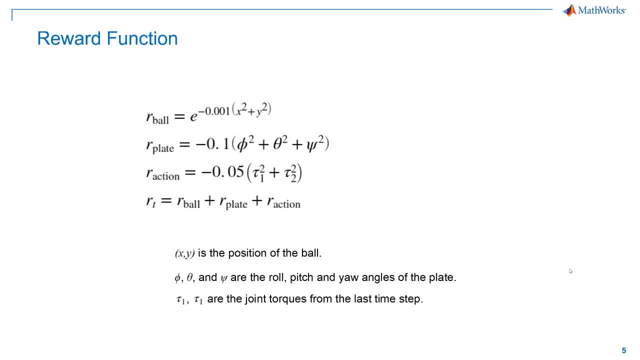 This reward could be a sparse value at any particular state, but we can improve the reward by providing a shape in the form of a non-linear function. In this case, we use a Gaussian function to reward the agent, as the x and y distances of the ball goes to zero. 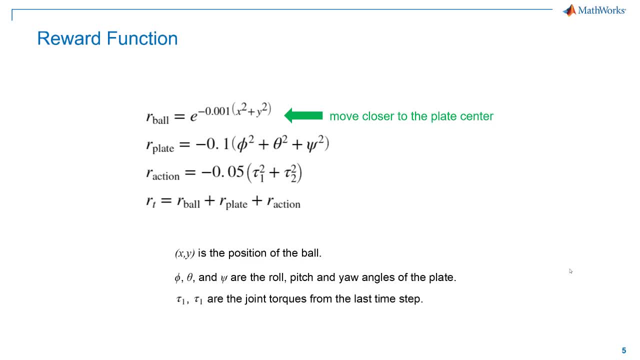 After you train the agent a few times, you will find that a well-shaped reward helps in improving training convergence In addition to moving the ball to the center. we also want to avoid a non-linear function, Since the reward is well created with such a well- 블�base function. the white and 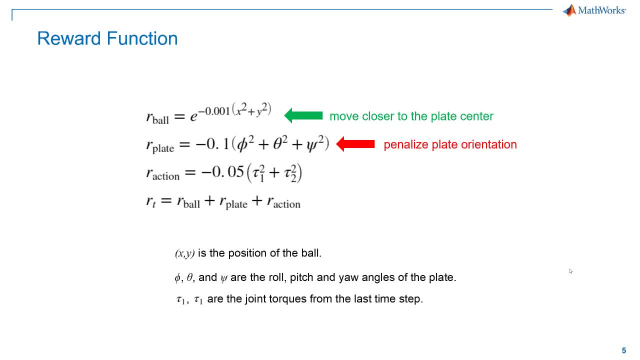 72 degrees partner we goals given becomes breakoutury relative In contouring. we also provide a grade value with weight score value and value devote per cent to the resultingither reward, in addition to being equal to 1 and 3.. 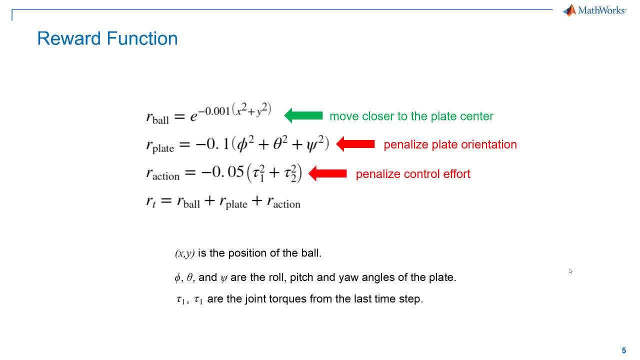 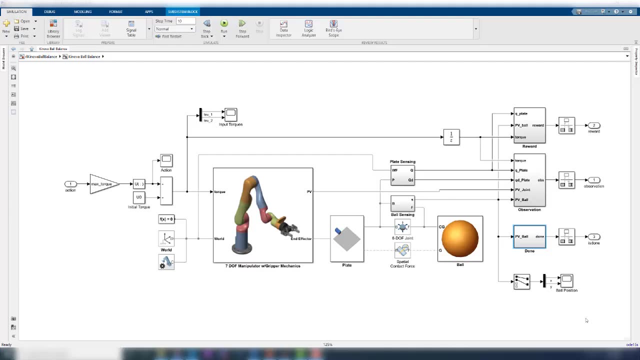 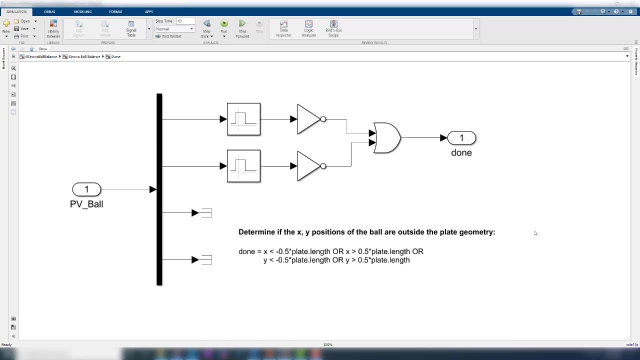 The score value is given by theici and the total reward useful during this particle control function. To add to this, we have two things: 1.. 2. the overall reward. The final set of signals from the environment is a logical is done signal that determines when the simulation should be terminated. 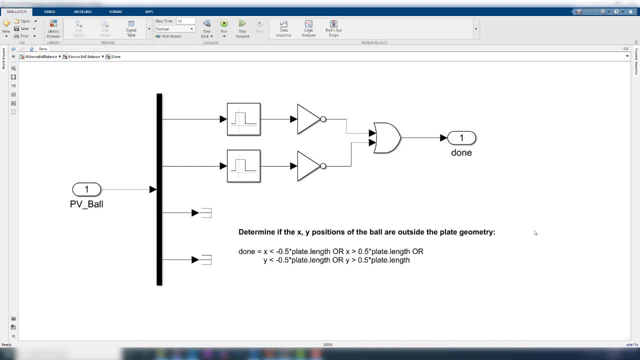 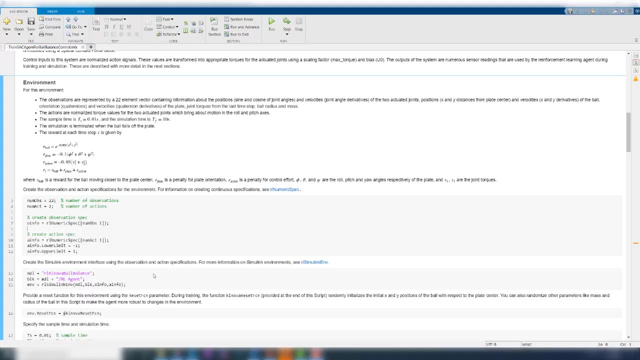 Termination could mean the system has reached a bad state and it does not make sense to simulate further. In this case, we terminate the simulation when the ball falls off the plate by comparing the XY coordinates against the plate boundaries. Let's go back to the live script to create a reinforcement. 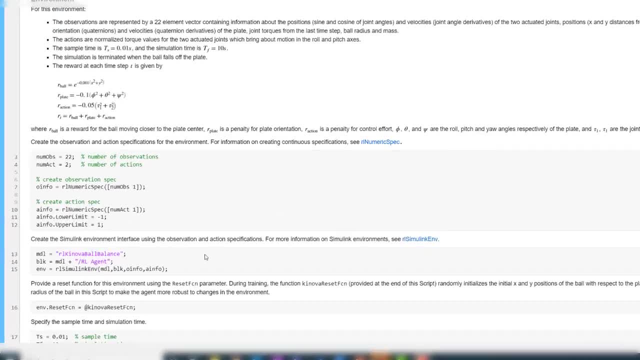 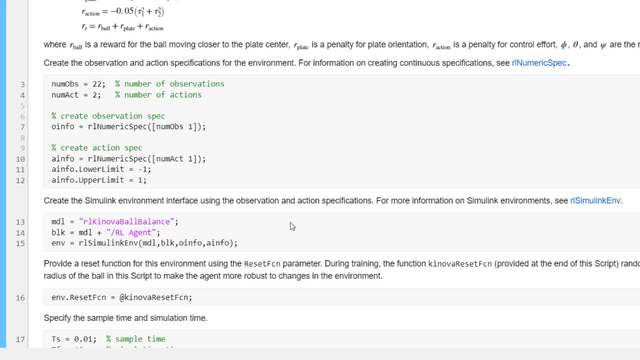 learning environment from the Simulink model. First, you will need to create specifications for the inputs and outputs. Since the observation and action spaces are continuous, in our case, you can use the RL numeric spec function to create the specifications as shown here. Once you have the specifications created, 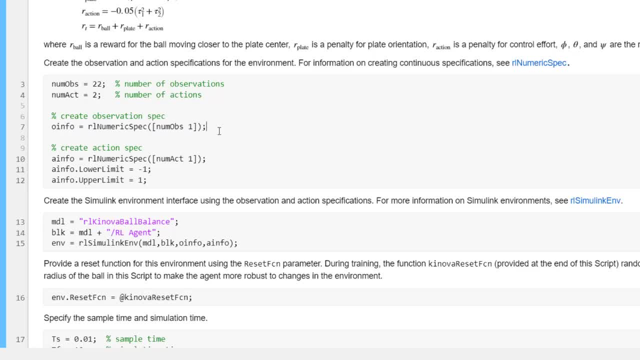 you can create an environment as the simulation model creates a simulation model. to create a new environment object using the RL Simulink ENV function, as shown here, You will need to specify the Simulink model name, the block path through the RL agent block and the observation and action specifications that we created before. 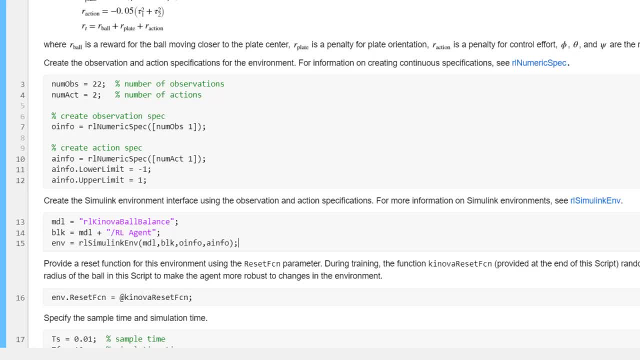 One important aspect of training an RL agent is domain randomization. You can randomize the Simulink environment at the beginning of each training episode by providing a function handle to reset the environment, as done here. This randomization can help the agent learn a policy that is robust to variations within. 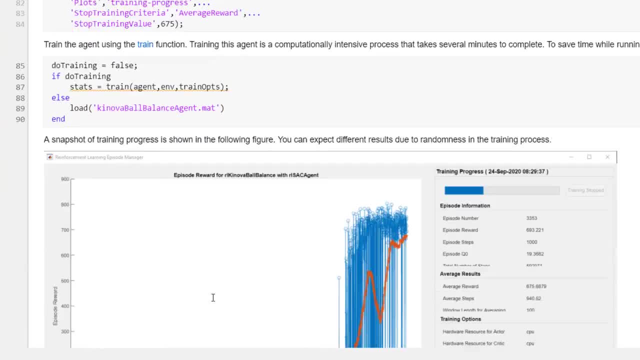 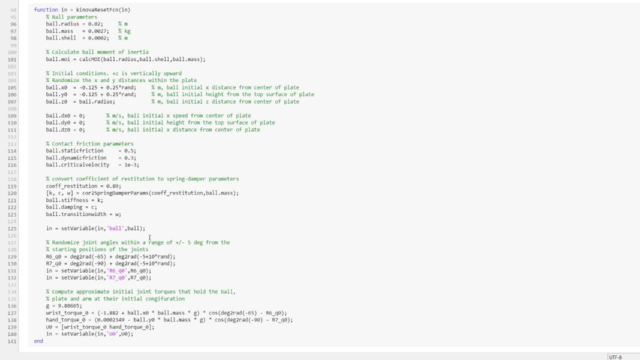 the environment. Scroll down to the end of the script to view the reset function. Over here there are some parameters that may be important for randomization, such as the ball physical parameters, then the initial joint angles and the initial torques. 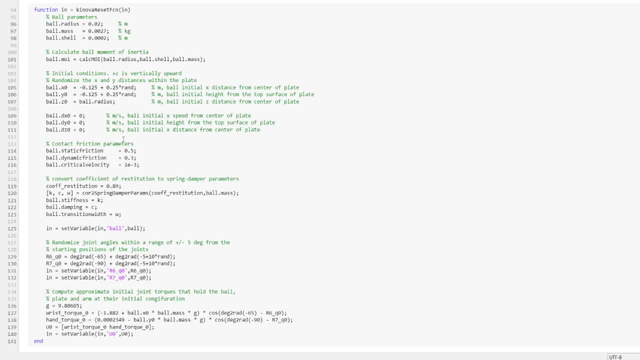 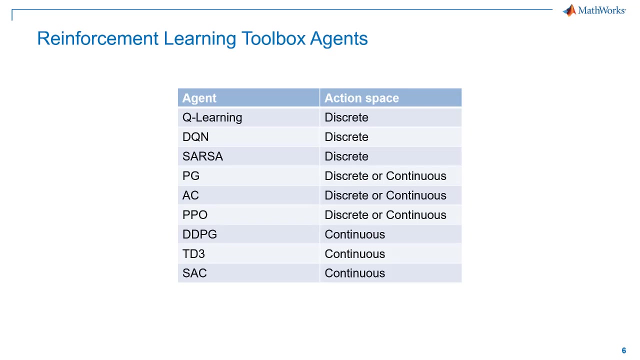 You can introduce randomness in these parameters as you like, but for now, let's focus on randomizing just the initial positions of the ball and then keep the other parameters constant. After creating the environment, the next step is to create a reinforcement learning agent. 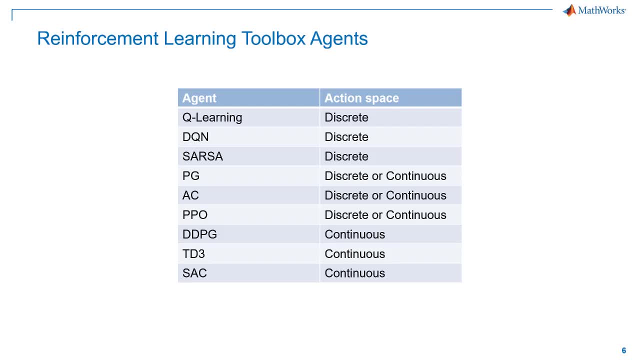 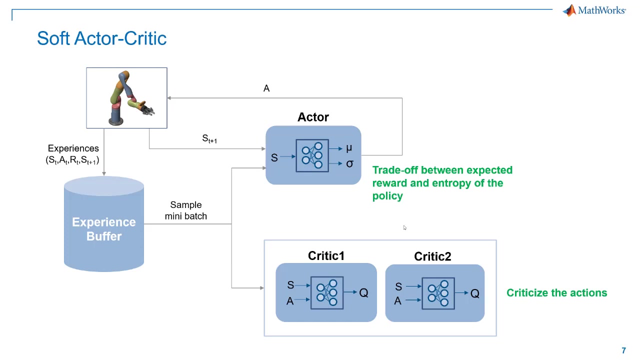 in MATLAB, There are many algorithms to choose from in the reinforcement learning toolbox. These algorithms work on either discrete or continuous action spaces, or both. For this tutorial, you will be using the Soft Actor Critic agent, which supports continuous action space. Here is a high-level explanation of the Soft Actor Critic algorithm. 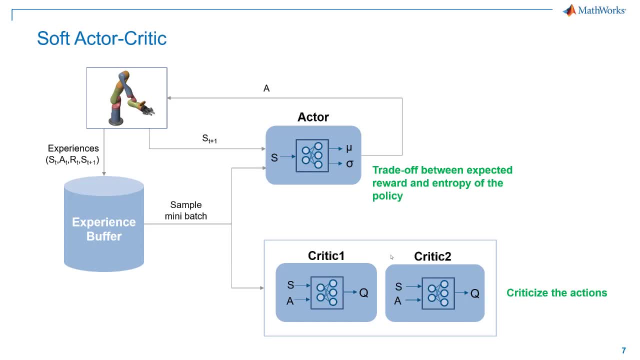 The items in blue represent the major components of the agent. An experience buffer is used to store experiences from the agent-environment interactions and the agent learns by using sample data from this buffer. The learning algorithm for this agent follows the actor-critic approach, with one actor and. 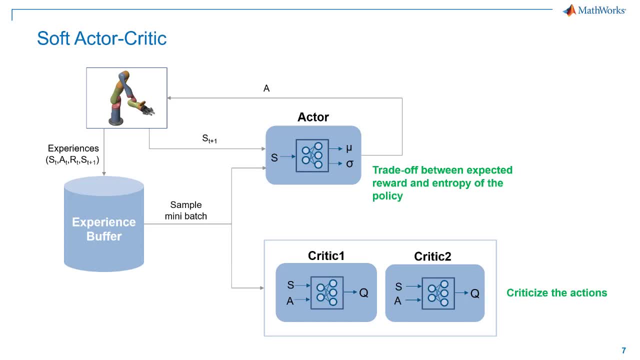 two critics, Each of which are represented by neural networks. The actor looks at the environment states and selects the actions based on a mean and variance output from the network, as shown over here. This mean and variance defines the stochastic policy of the actor and is used to compute. 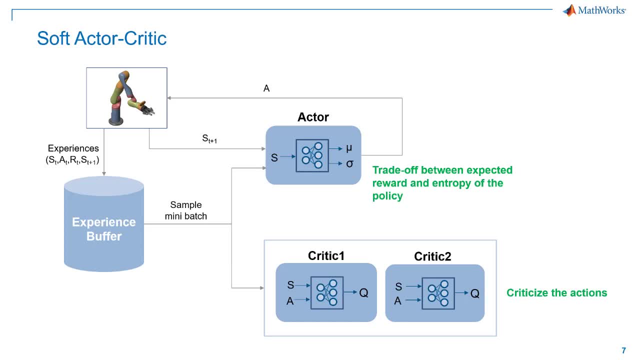 the agent's actions During training. the weights of the actor network are updated by a trade-off between the expected reward and the entropy of the policy. The critics kind of sit behind the scenes. You can see that the actor's actions are based on the expected reward and the entropy of. 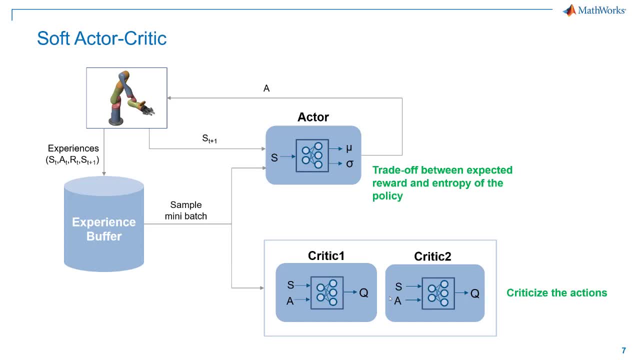 the policy. You can also find the actor and criticize the actions, whether they are good or bad. Their weights are also updated periodically. The algorithm uses multiple critics to reduce over-estimation of the Q function. You can find more information on the Soft Actor Critic algorithm towards the end of. 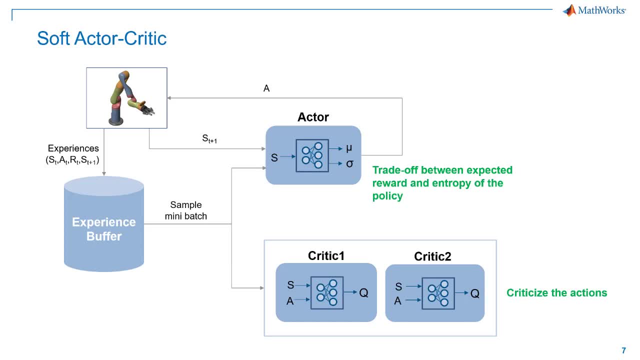 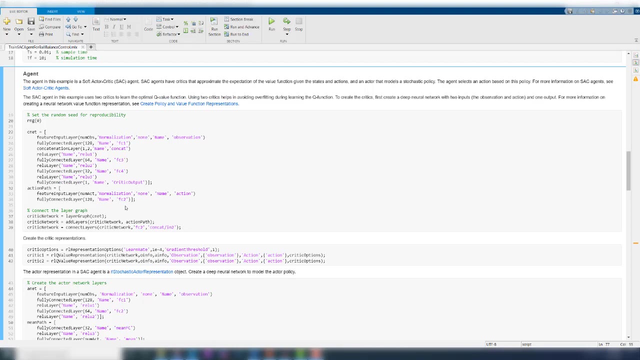 this tutorial, but for now, all you need to do is to create these neural networks in MATLAB. Everything else will be handled by the toolbox. Now we are back to the live script again. You can create the neural networks by running the code in this section. 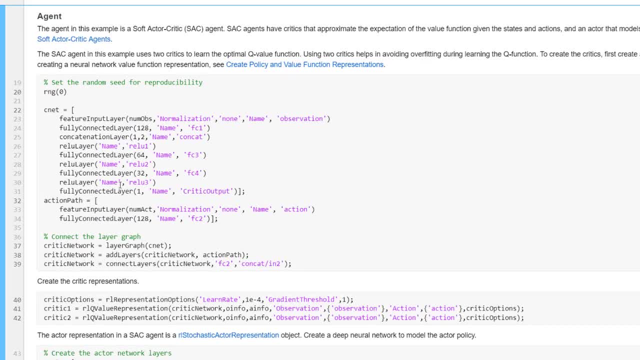 As shown here, the critic networks consist of a few fully connected layers with value layers in between. The inputs to this network are the observations and actions of the agent and the output is the Q function value. You can use the same critic network to create the two critics. 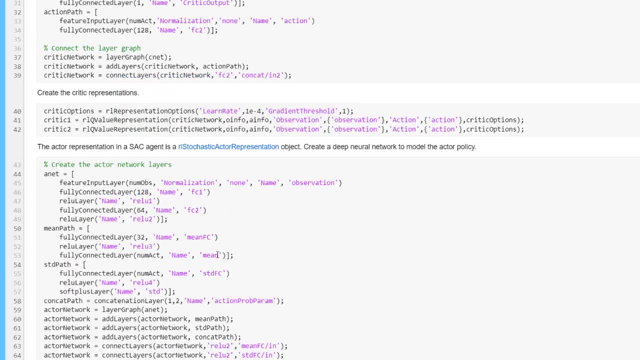 The actor is also modeled in a similar way. The actor is also modeled in a similar way. The actor is also modeled in a similar way. It takes observations as inputs and outputs, the mean and variance of the policy distribution. After creating the actor and critics, you can create the agent using the RLSACAGENT function. 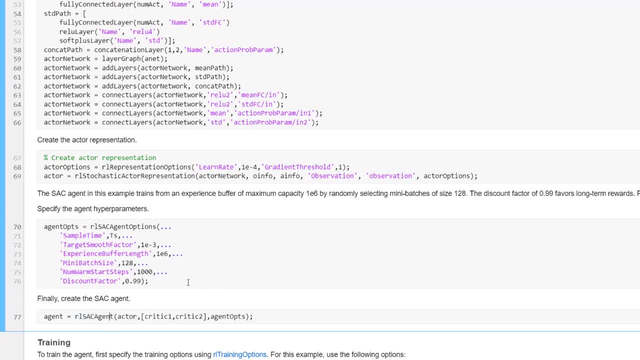 as shown here. Most of the hyperparameters of the agent are kept to their default values as shown here, So you need not worry too much about changing them for this tutorial. For a full list of hyperparameters, you can click on this link, which will take you to. 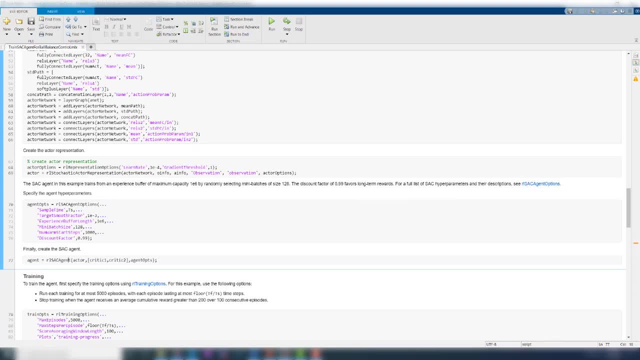 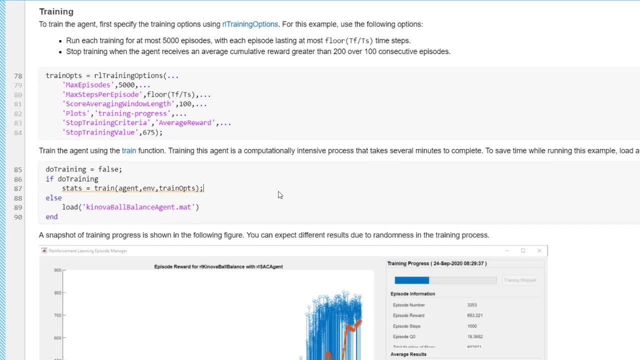 the MATLAB documentation. Thank you. Once the agent is created, the final step is to train the algorithm using the train command. You can specify a few training options, such as how long the agent is going to train and what is the stop value for training. 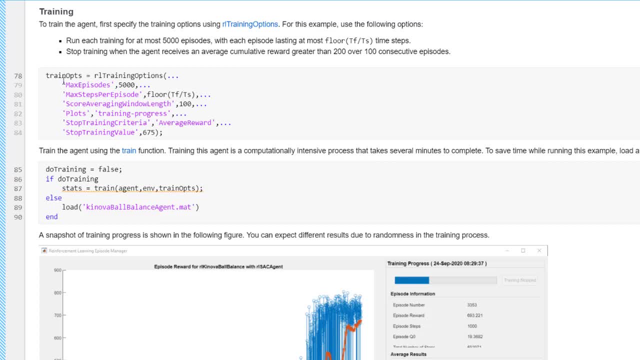 For example, you can set the maximum number of training episodes, as shown here, and then the maximum steps for training episode. Another important parameter is the stop training criteria. In this case, we stop the training when the average reward over the last 100 episodes reaches the value of 675 or more. 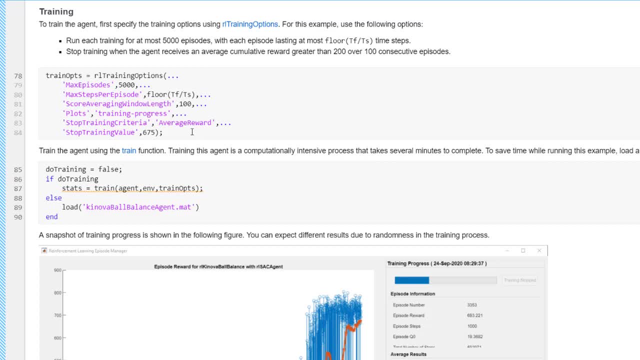 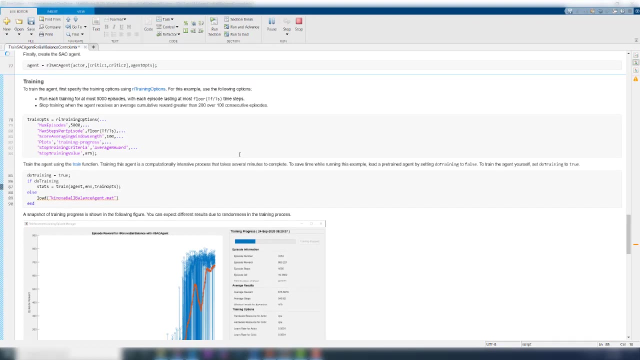 This value was obtained after analyzing the agent's performance for a few training iterations. To start the training, you can set this doTraining flag to true and execute the code in this section. The software will take a few seconds to set up the training and will launch an episode manager. 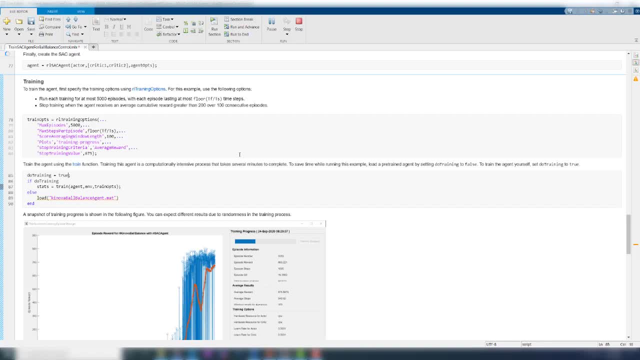 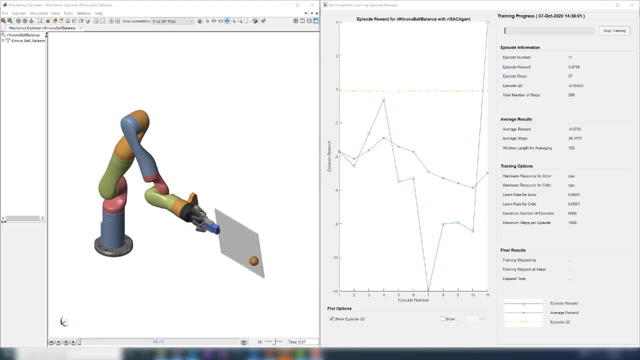 After launching the training, you can view the training progress from the plot, as well as see the animation in the Mechanics Explorer window. You can see here that the agent is trying to balance the ball, but failing most of the time. This is expected because it is towards the beginning of training and the agent has not learned much. 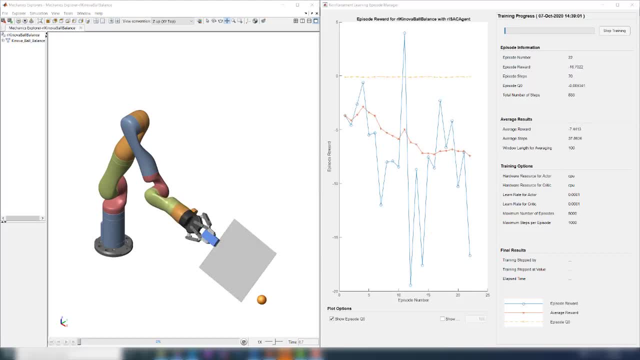 You will also see from the plot that the agent does not receive too many rewards per episode. In the figure, the blue line represents the episode reward and the red line represents the average reward over a window of 100 episodes. The yellow line represents the expected long-term reward. 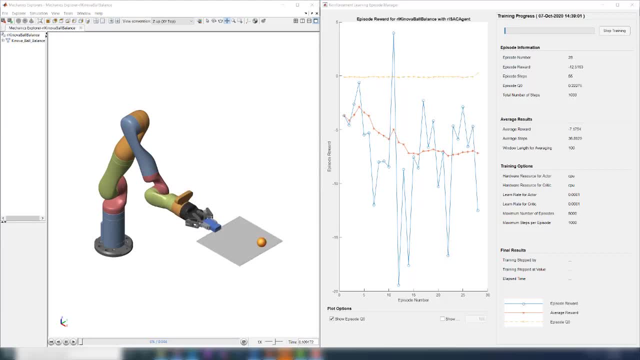 As the agent learns from experiences, you will see that the rewards will increase and converge to some value. At that point you can stop the training and view the agent's performance. To stop the training, you can simply click on the stop training button over here. 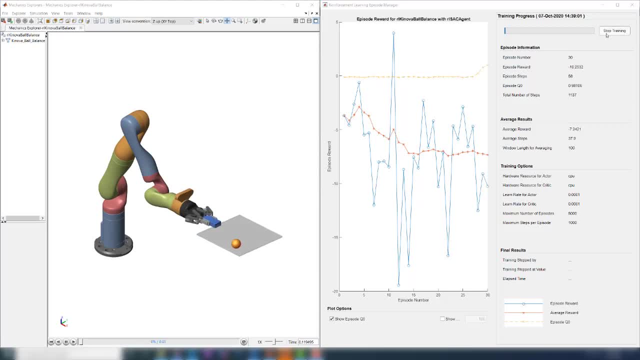 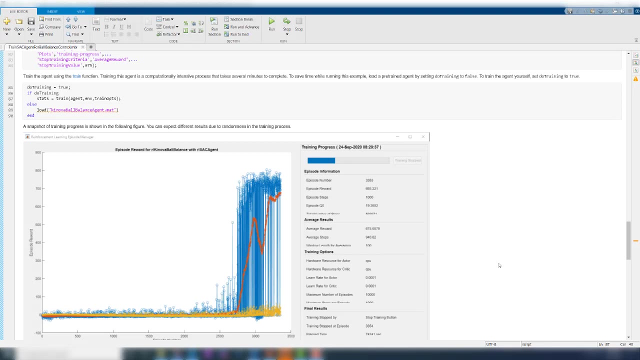 In the interest of time, let's stop the training. Let's stop the training and continue with the live script. A snapshot of a completed training session is shown in the figure here. This will give you an idea of what to expect in the training process. 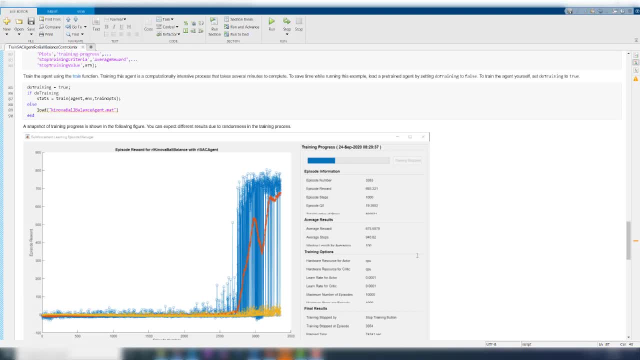 For this particular training, the agent reached the average reward of 675 after about 3,300 episodes. It took about 20 hours to complete. Depending on your system specifications, the training may take lesser time or more. Also, since there is randomness in the process, your actual results may be a little different from what is shown here. 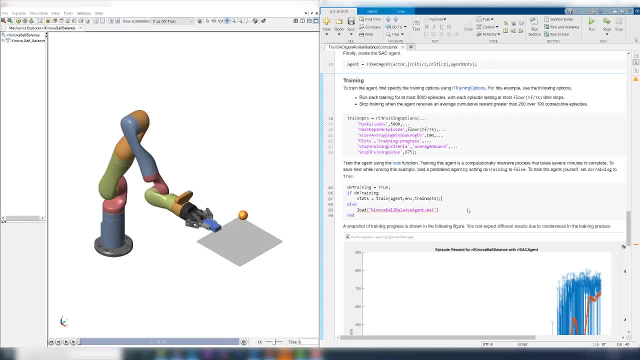 Let's load a pre-trained agent now to view its performance. You can set the DoTraining flag back to false to load an agent saved in a mat file. You can run this section again to load the file. After loading the agent, scroll down to the top of the screen. 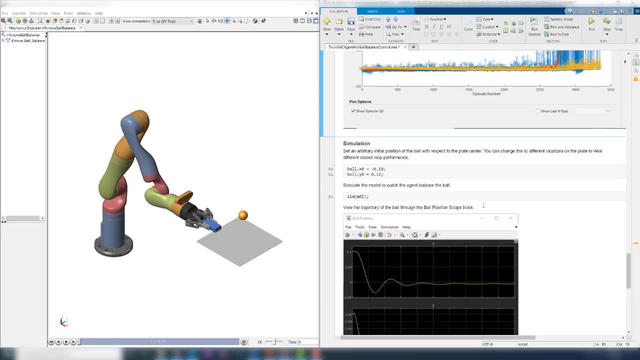 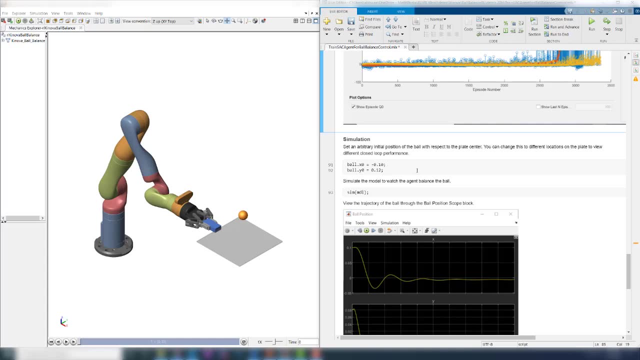 You can see that the agent has been loaded. After loading the agent, scroll down to the simulation section. Here you can set the initial position of the ball to your liking and simulate the model, This time with a trained agent. Over here the initial X and Y positions are set to some non-zero values. 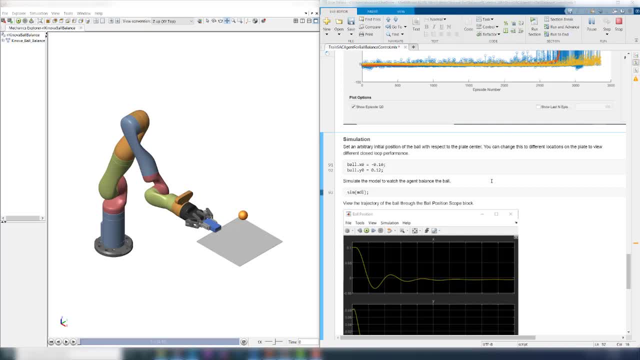 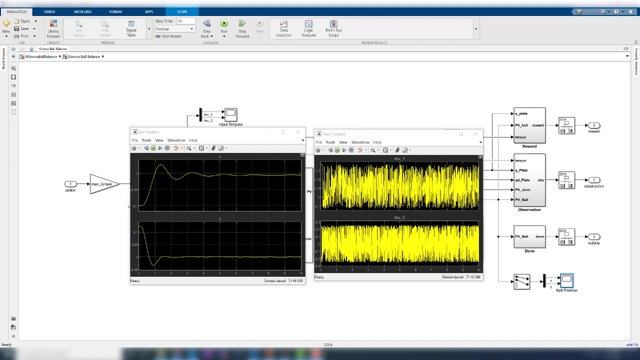 Let's run this section. You can now see in the animation that the agent is able to center the ball successfully. You can try simulating a few different times with different initial conditions. Going back to the Simulink model, you can view the trajectory of the ball and the control inputs through the scope blocks.